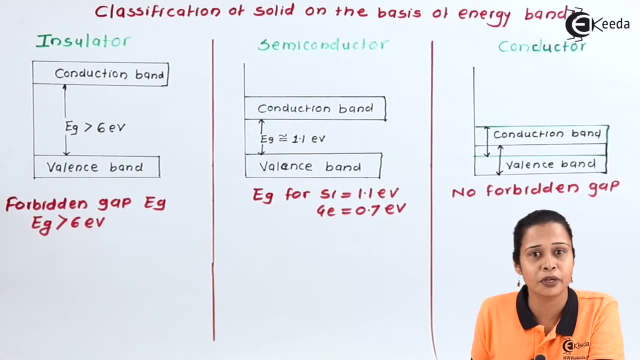 considering any insulating material, for example rubber or wood. Now we know all the electron in that material is tightly bound with the nucleus, So there are no free electron for the conduction. But suppose we are applying more than 6 electron holds energy to the material. What happened with? 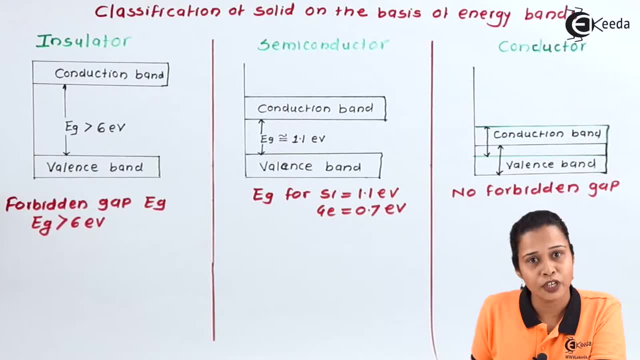 that Then- or we can say in terms of heat, suppose we are applying more heat to the material, still there is a no possibility of the free electron Means. still that insulator cannot convert into the conductor, Because if you give more heat or more electric energy, then that rubber or wood will get spoiled. The 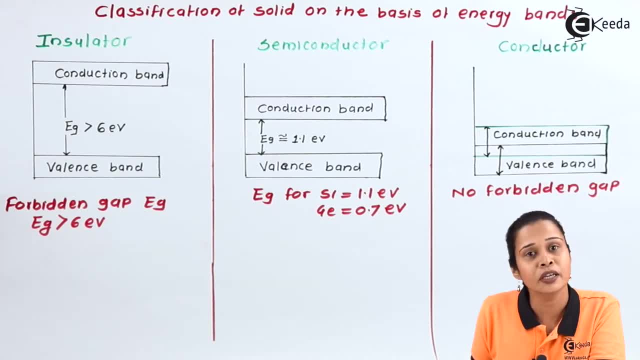 structure will destroy but it will not convert into the conductor. So the conversion of insulator to conductor is quite difficult, even if you are applying more amount of energy than the band gap energy. In case of conductor we can say there is overlapping of the conduction and valence band. 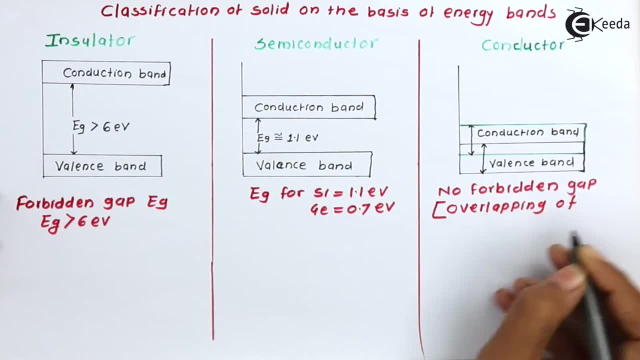 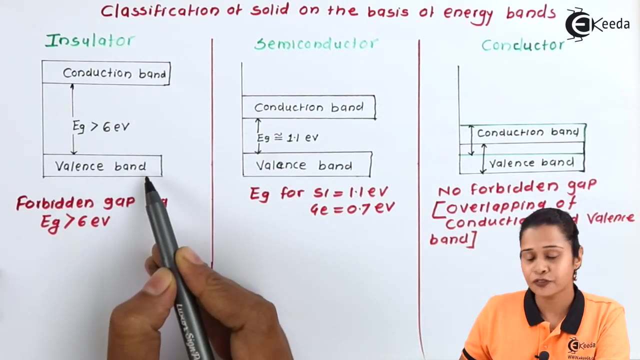 No, badlyって anrill토. by this double solution nella in this case it won't work here. Now second point: here, In case of insulator, valence band is fulfilled and conduction band is empty. Becausein case of insulator we don't have free electron, means our conduction band is emptyBut valence band is fulfilled. 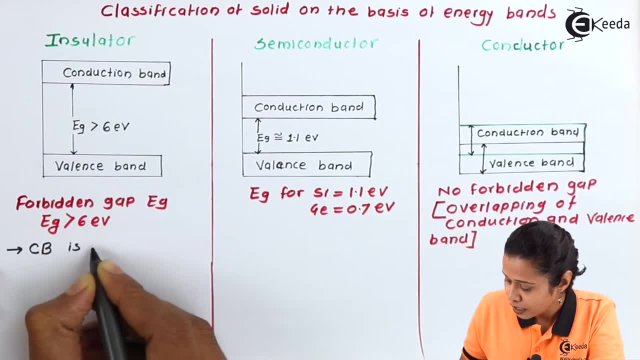 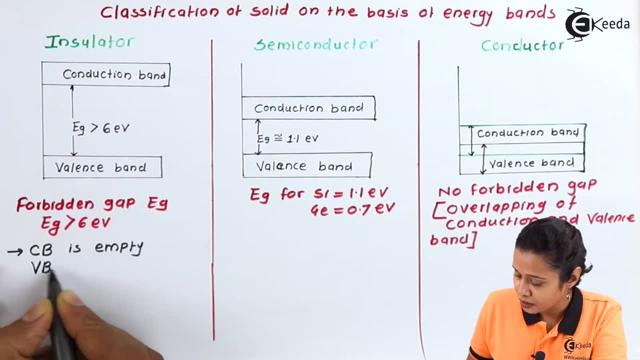 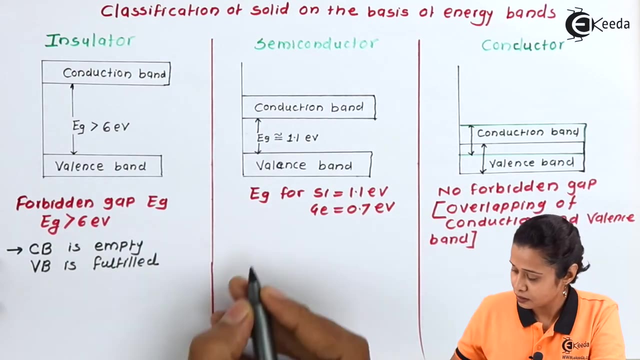 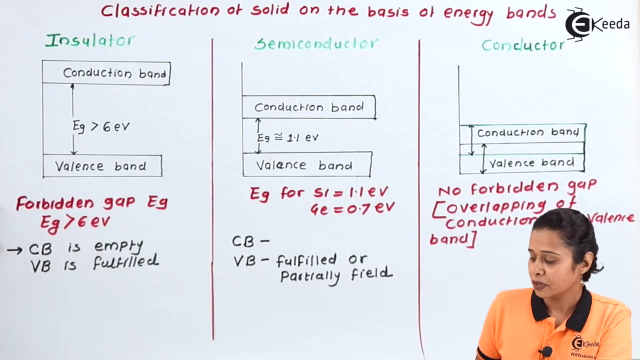 conduction band that is CB is empty and valence band that is VB is fulfilled In case of semiconductor conduction band and valence band in case of semiconductor valence band is fulfilled or partially filled Means suppose the semiconductor material is below room temperature. means the temperature.